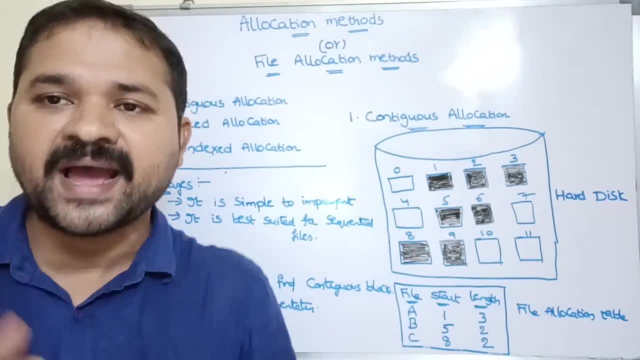 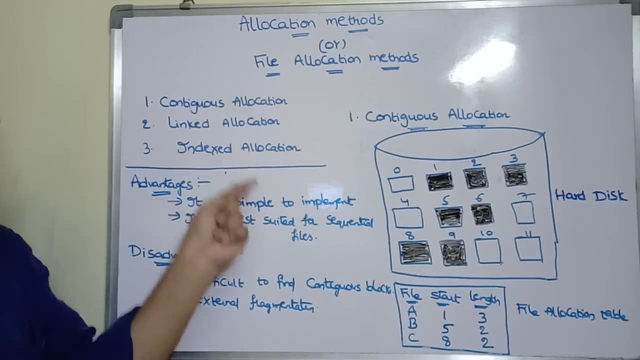 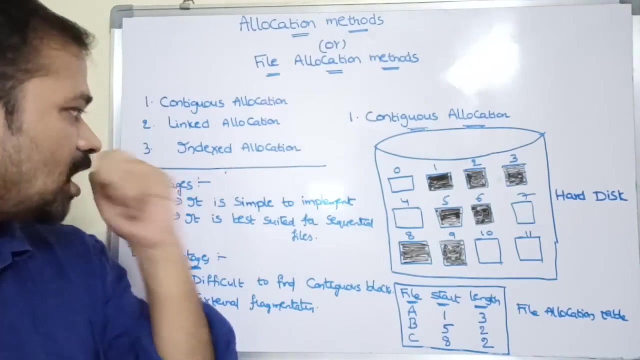 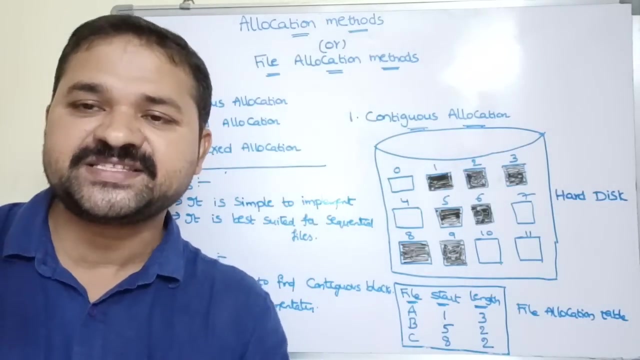 So by keeping these two goals in mind, operating system allocates space for the files. There are three types of file allocation methods are available. First one is contiguous allocation. Second one is linker allocation. Third one is indexed allocation. So let's see the first one, contiguous allocation. The name itself specifies the meaning. So in this approach, a set of contiguous blocks will be allocated. 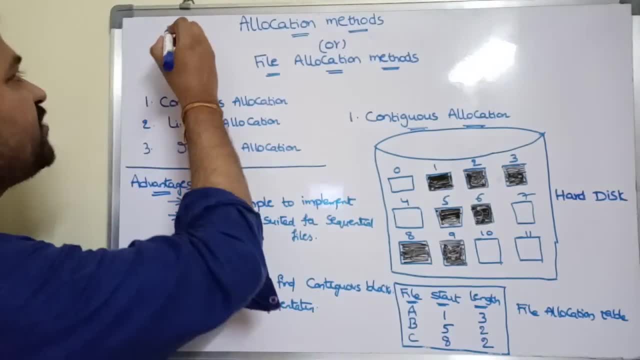 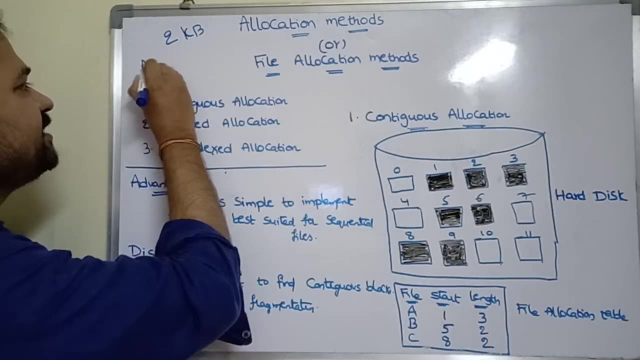 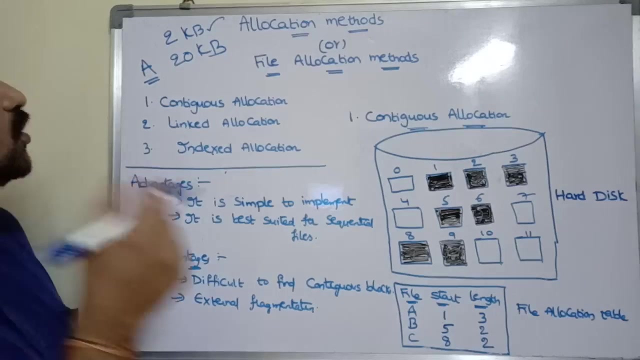 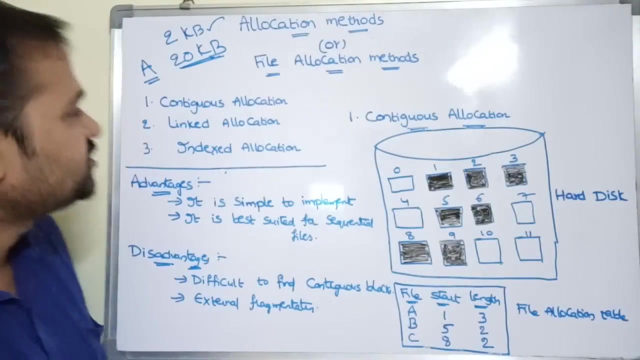 For a file. Let here: let the size of a block is 2 KB. Size of a block is 2 KB. Let file name is A Let size of a file is 20 KB. So what is the size of each block? 2 KB Various. what is the size of our file? 20 KB. So if you use this contiguous allocation, then totally 10 blocks needs to be allocated for A. 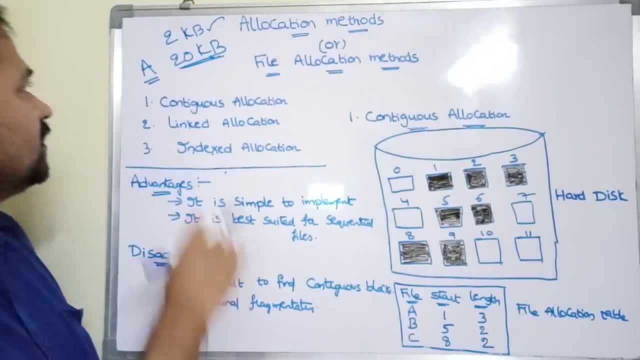 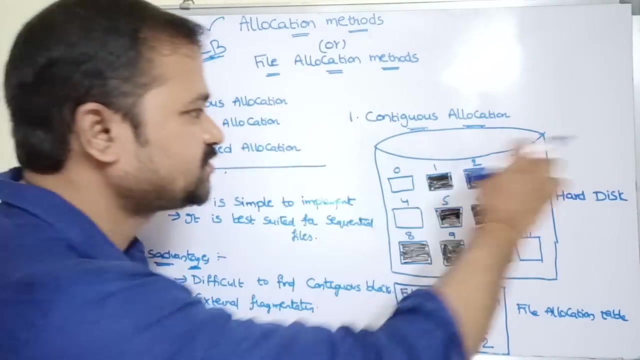 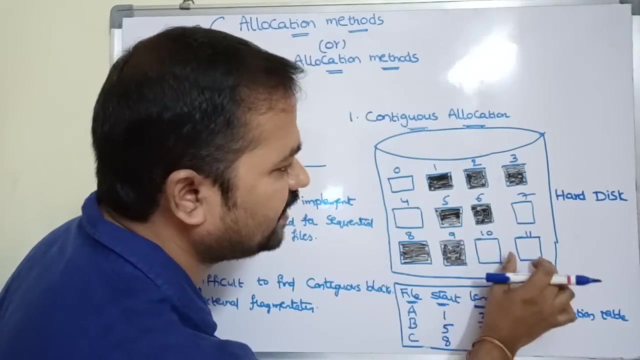 Let us assume that the size of each block is 1 KB, Then 20 contiguous blocks needs to be allocated for file name. So this is about contiguous allocation. So this is the hard disk, as well as this one is nothing but file allocation table. So in hard disk we have totally 12 blocks, ranging from 0 to 11.. 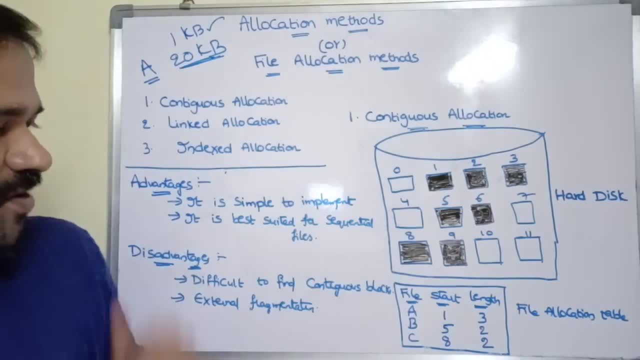 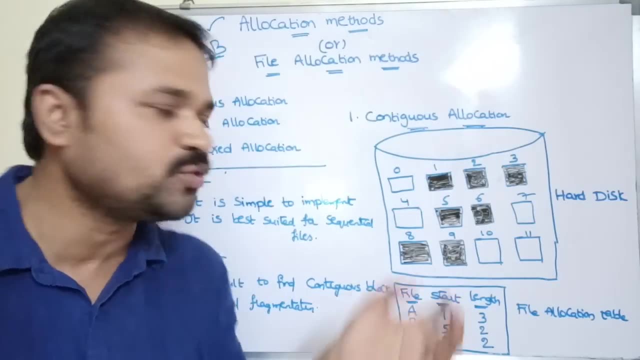 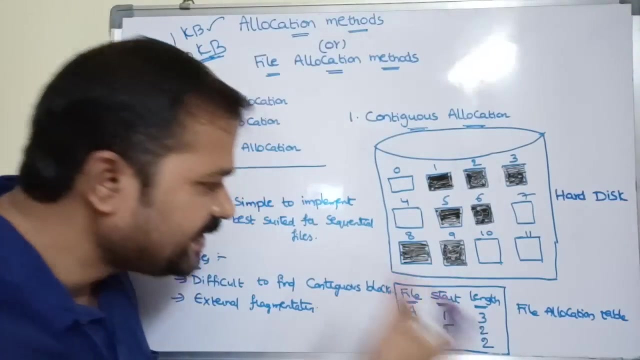 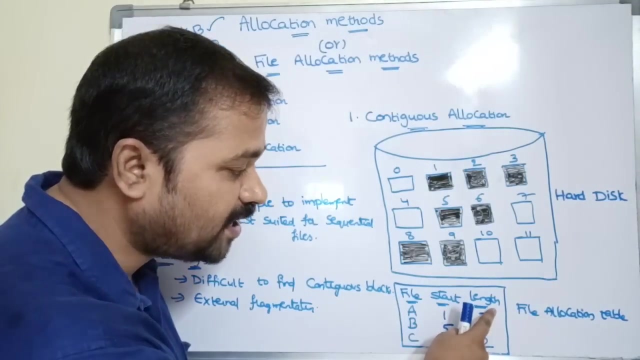 Okay, So totally, we have how many blocks? 12 blocks. Okay. So this is nothing but file allocation table. So file allocation table contains the information about each and every file that is stored in the secondary storage. that is nothing but hard disk. It mainly contains three columns. The first column is name of the file. Second column is starting block number And the third column is length of the file. Okay, 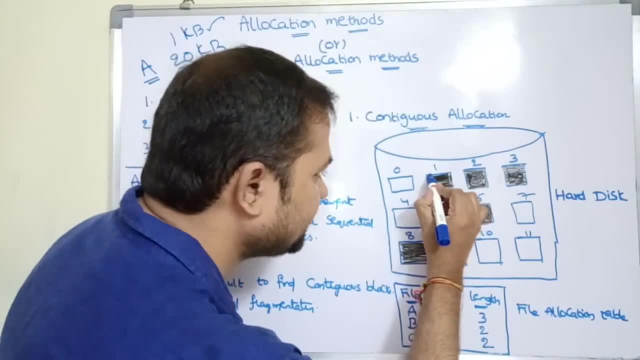 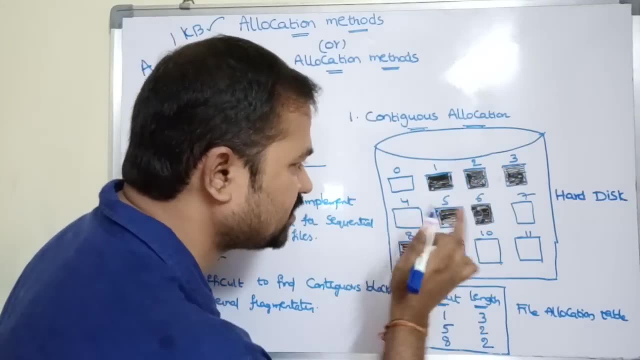 First column is A Starting block is 1.. So that means this is that block And what is the length of this? A? 3 blocks, So 1, 2, 3.. 3 blocks, So file A is occupied by these 3 blocks: 1, 2, 3.. 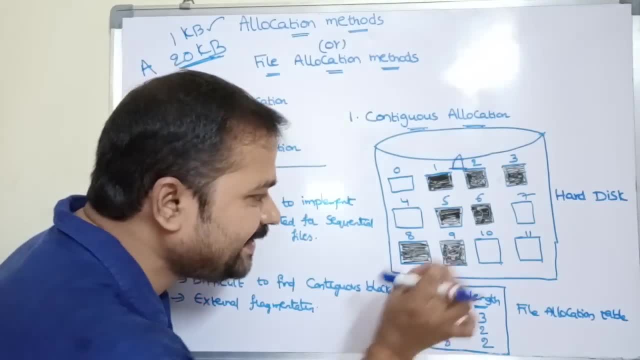 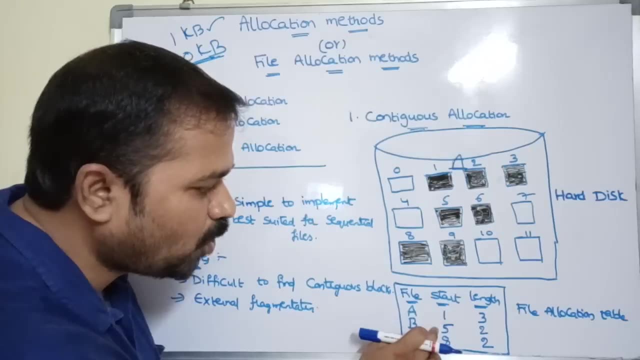 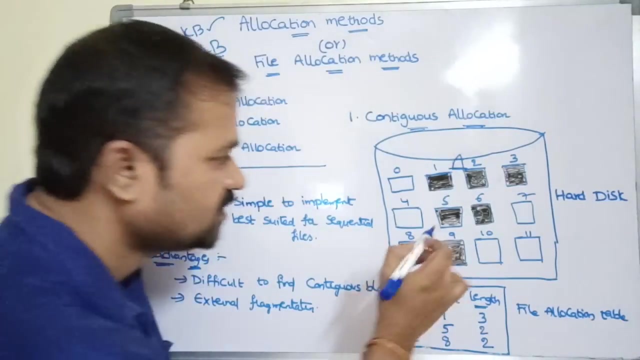 So for each file we can have a single entry in the file allocation table. Let us observe the second row. So name of the file is B, Various. the starting block number is 5.. So this is fit to black. what is the length of the file? two blocks so five, six, one, two say. these two are occupied by b. 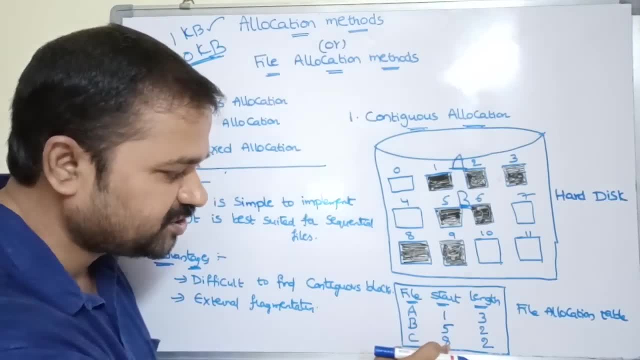 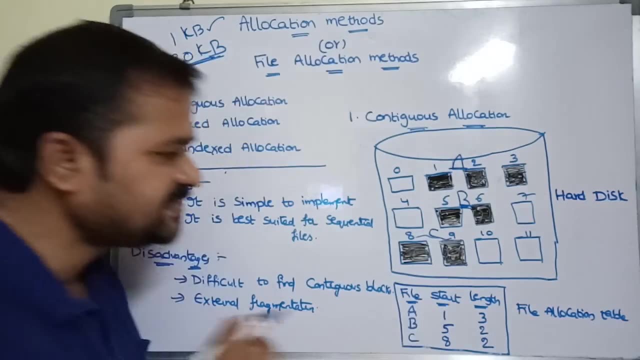 and next we have one more row that is about c information. the starting block number is eight, as well as what is the length of the file: two blocks. so these two blocks are occupied by c. so this is about file allocation table. so file allocation table contains the information about. 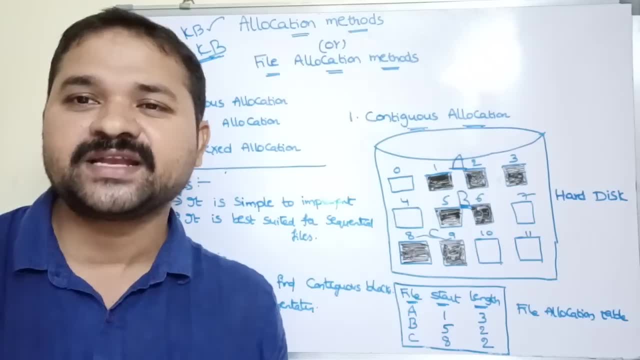 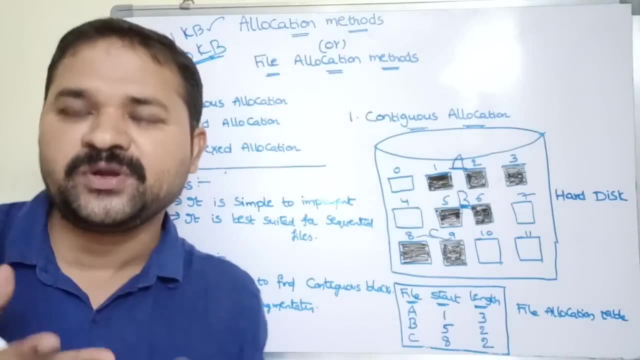 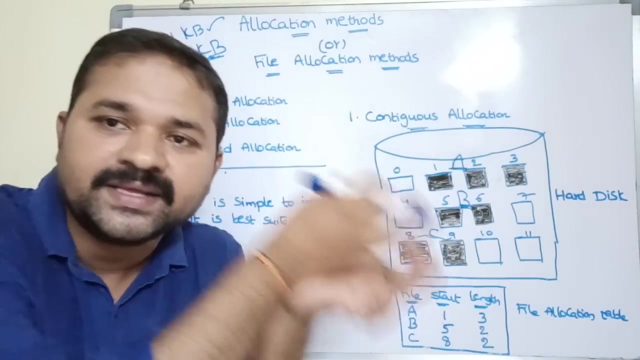 the files which are stored in the hard disk. and now let us analyze the advantages and disadvantages of this approach. the first advantage of this approach is it is simple to implement. why? because we need only a conjugate set of blocks, and in those blocks operating system allocates space for the files. so we can implement this approach in the easiest manner, and it is. 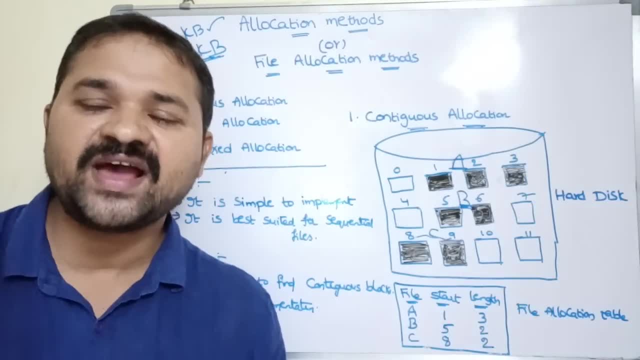 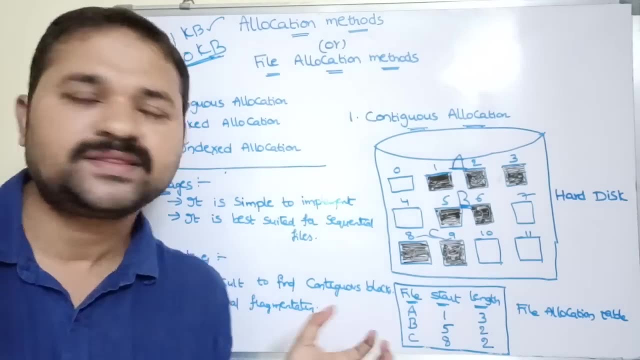 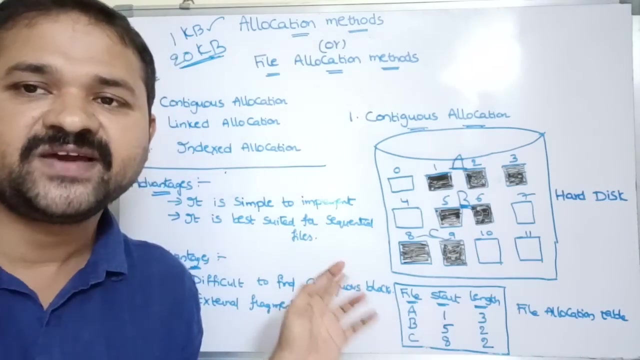 best suited for sequential file. so sequential file means the records can be accessed one by one. okay, so if we have sequential file accessing, then continuous allocation is the best one. why? because here also we are allocating memory in continuous blocks. sequential means accessing record by record. okay, so these are the advantages. 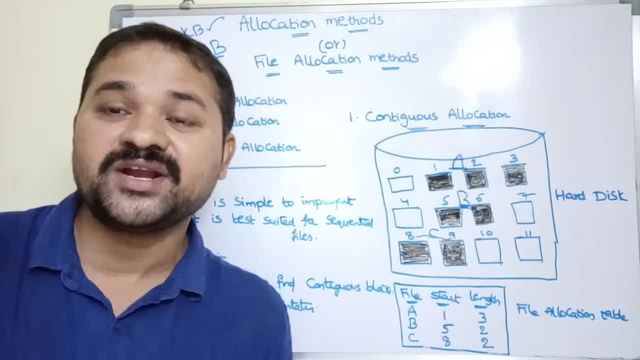 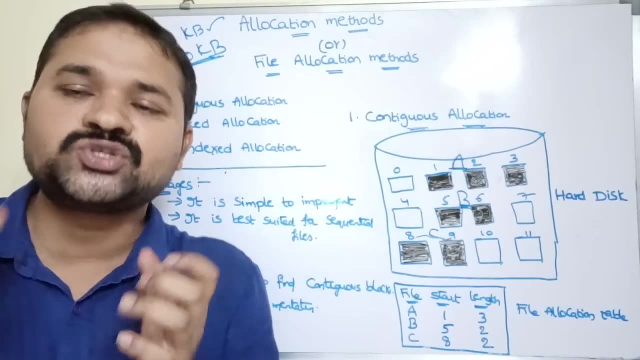 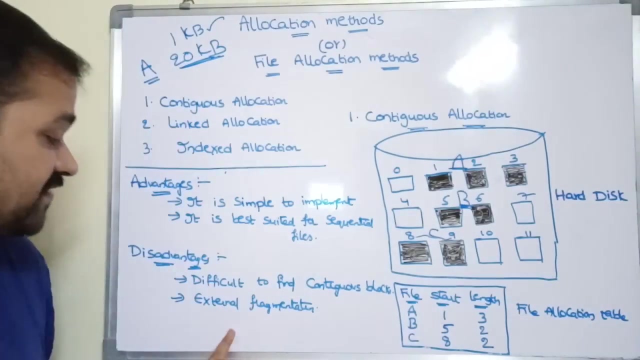 and the disadvantages are: difficult to find the continuous blocks, okay, so let us assume that we need to have 100 blocks, okay? so it is very, very difficult to find out 100 continuous blocks at once. so that is the first disadvantage here and the second disadvantage is external. 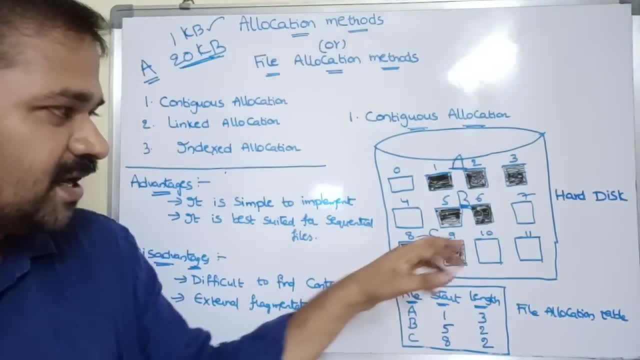 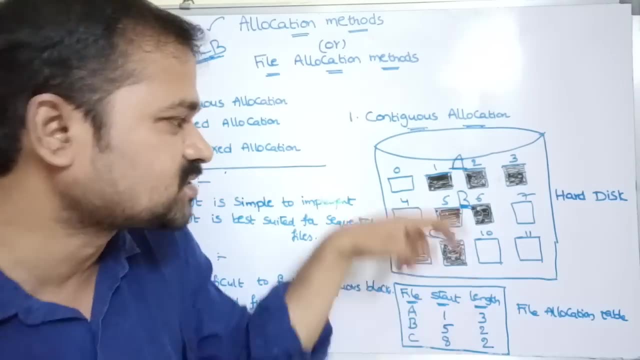 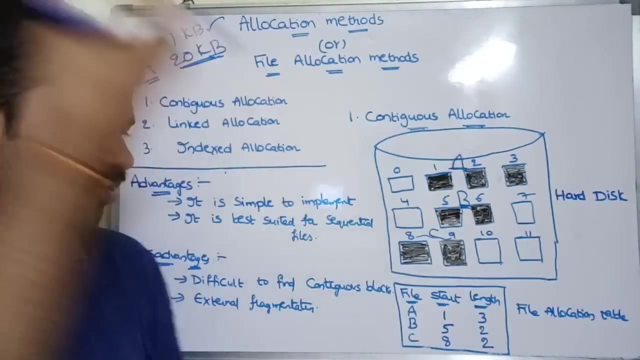 fragmentation. so we know what is external fragmentation and sufficient blocks are available in the heart disc, but they are available at different locations. the first two five blocks are available at once. second, uh, second five blocks are available, yet once thought, five blocks are available at one more location. like that, external fragmentation means sufficient free blocks are. 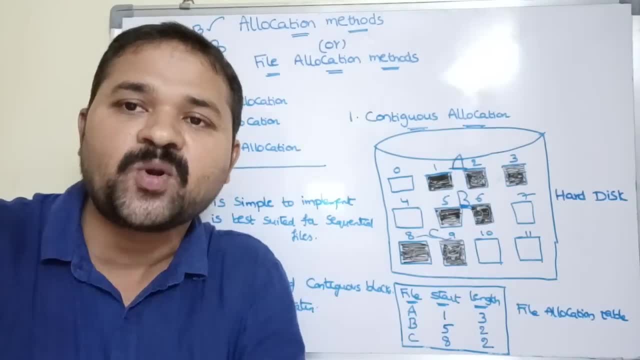 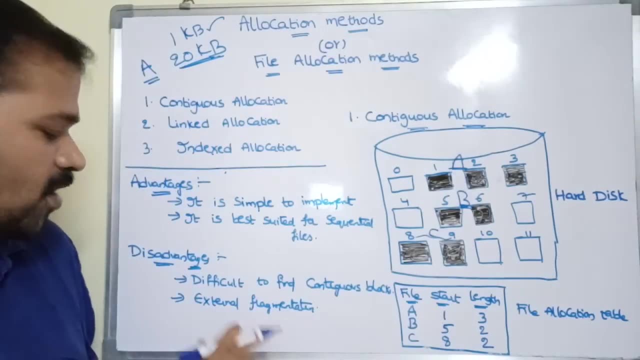 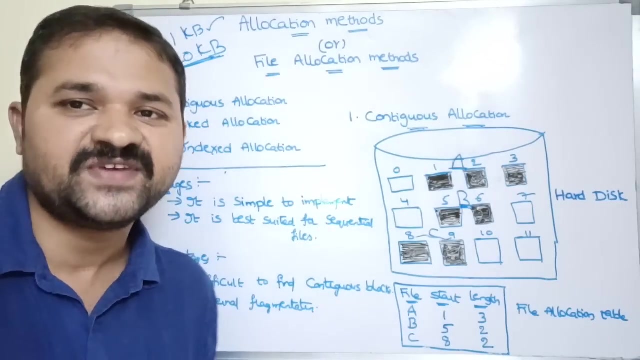 available, but operating system called allocates those blocks for the file. why? because those blocks are non-categorial. okay, so this is external fragmentation. so this is the problem here. we know that we can solve external fragmentation with the help of compaction, but compaction is very, very expensive approach. 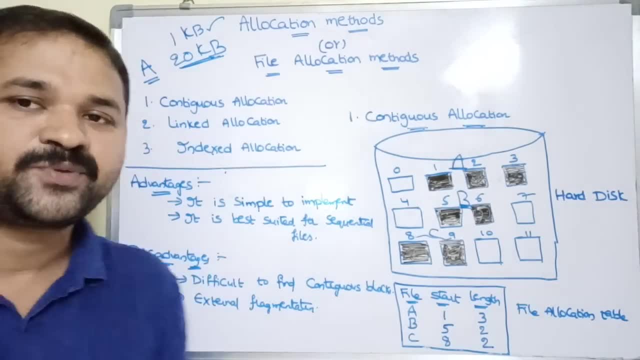 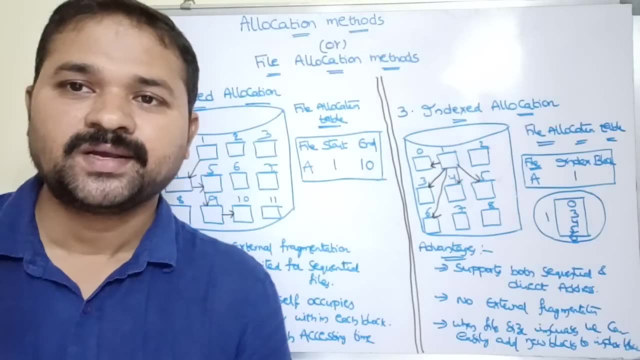 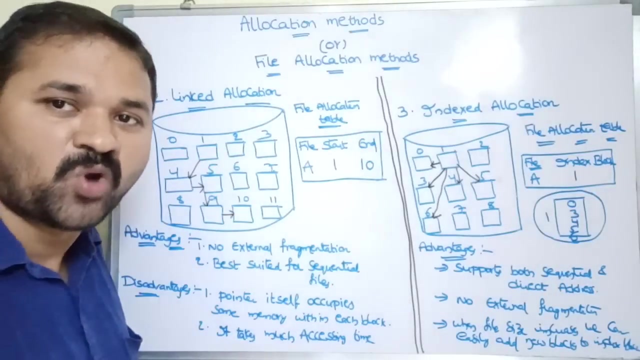 so, in order to overcome these problems, we can use the second approach, that is, link relocation. now let's see the second approach that is link relocation. it is based upon the link list. we know what is a linked list. here we can have a collection of blocks where in each block, we can 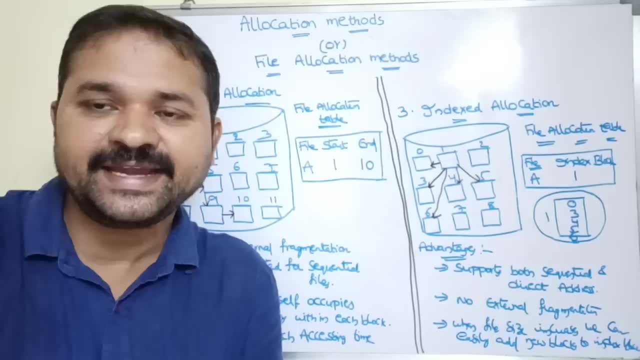 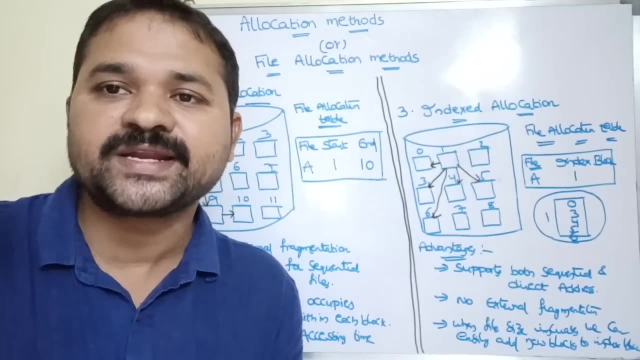 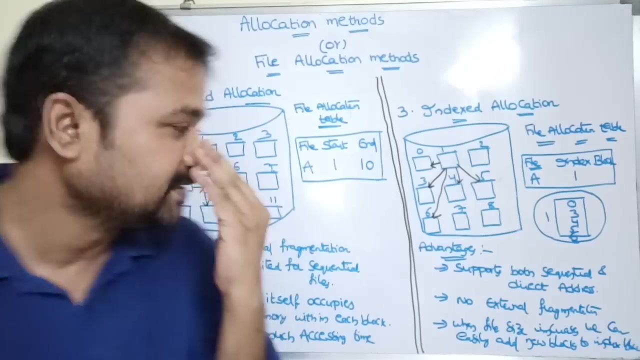 have a pointer field. so the first block pointer contains address of the second block. second block pointer contains address of the third block. third block pointer contains address of the fourth block, like that. so we can say that this approach is based upon individual blocks. so let us observe. 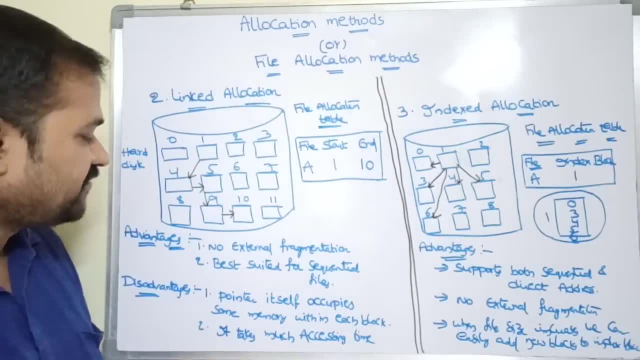 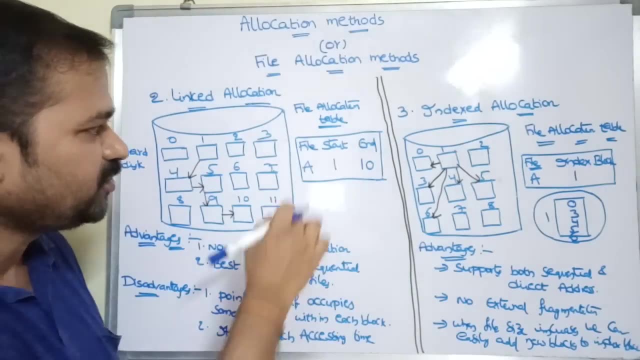 this diagram. so this is nothing but our secondary storage device, that there is nothing but hard disk. here we can have 12 blocks, from 0 to 11.. so this is nothing but file allocation table here. the file allocation table contains three columns. the first column is finding: 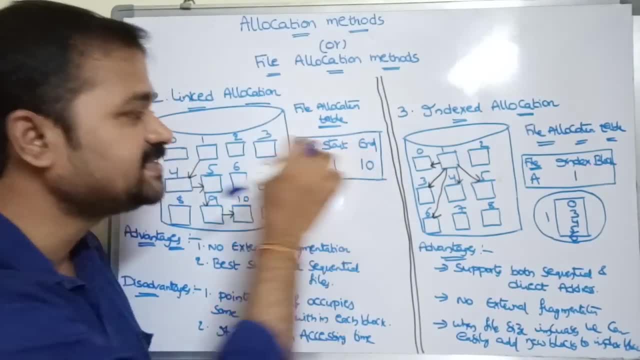 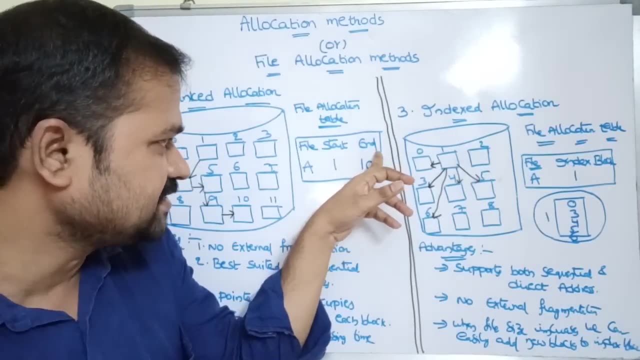 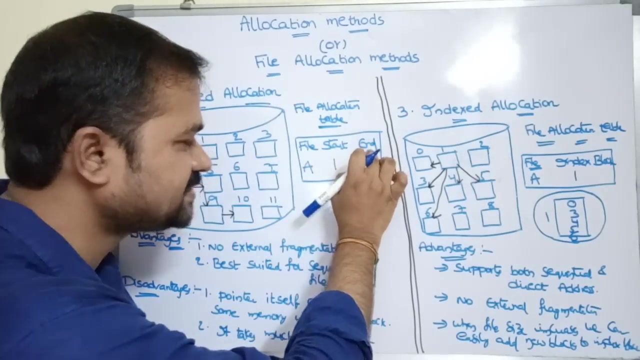 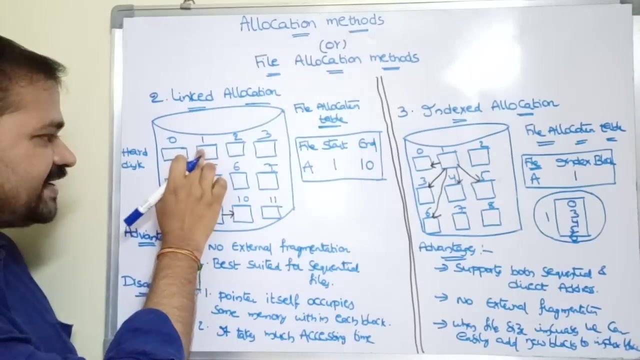 the second column is starting block number, whereas the third column is ending block number. various in contiguous allocation in file allocation table. the last column, the last one, is length of the corresponding file. so how many blocks does it occupy? various. here the third column is ending block number. so here name of the file is a. so what is the starting block number? so this one, so this one. 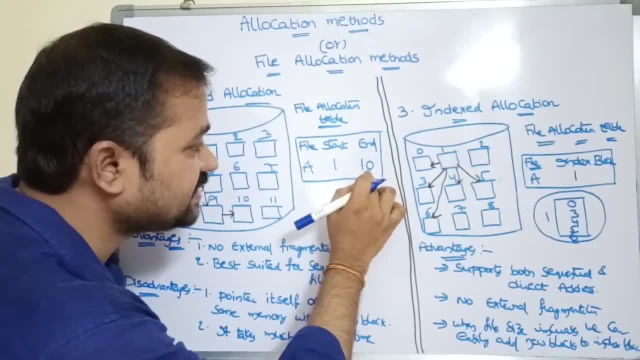 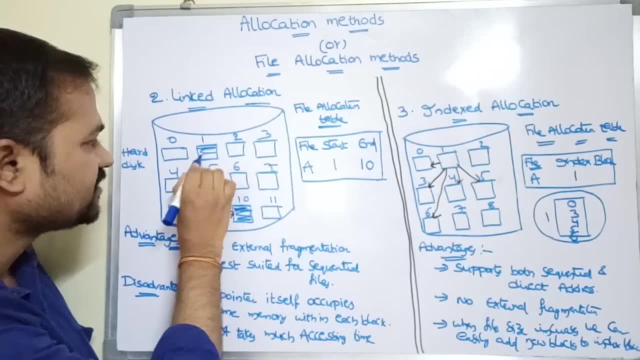 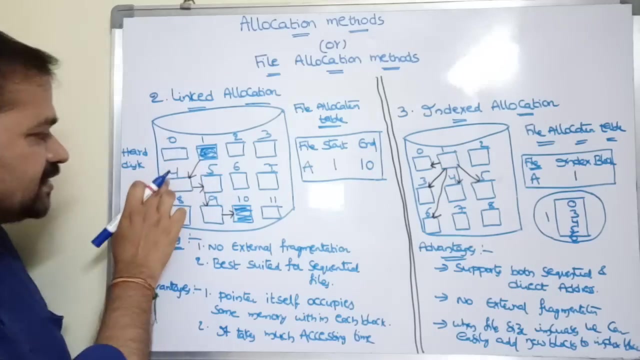 is the starting block number, whereas ending block number is nothing but 10.. so this is nothing but our last block, whereas this one is nothing but our starting block. okay, so this block contains a pointer. so this pointer points to the address of the next block. that is nothing but fourth block. 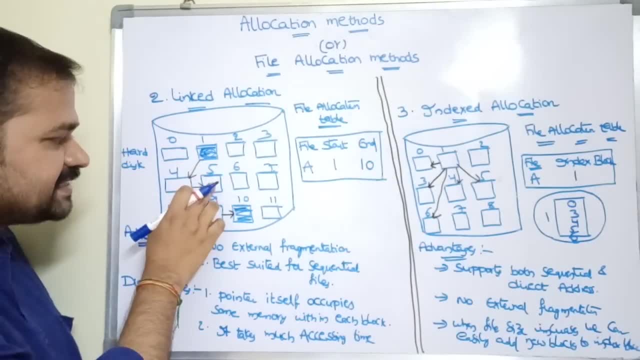 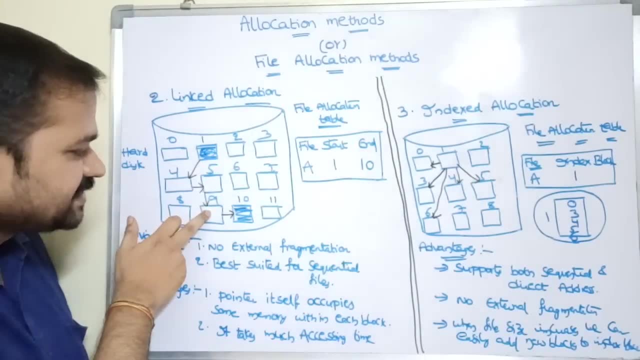 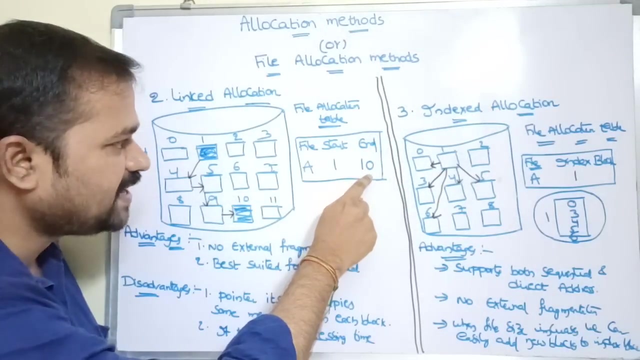 next, this block contains address of its next block. that is nothing but fifth block. Next, fifth block contains a pointer. It contains address of next block. that is nothing but ninth block. Next, this block contains address of its next block. that is nothing but tenth block. So here, what is the last block? here, 10 is the last. 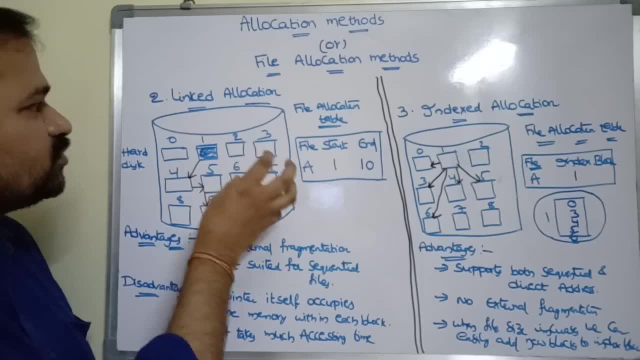 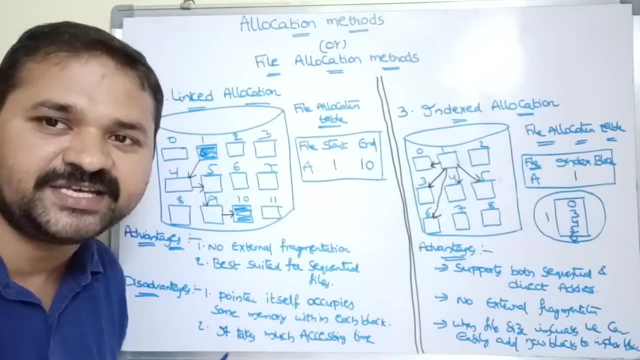 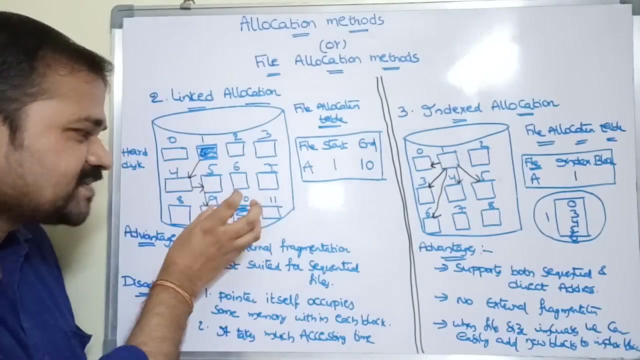 block here. So in this way we can allocate memory to the file with the help of a link list. Let us see the advantage here. The major problem with contiguous allocation is it suffers with external fragmentation, Whereas here external fragmentation does not arise here. Why? Because whenever there, 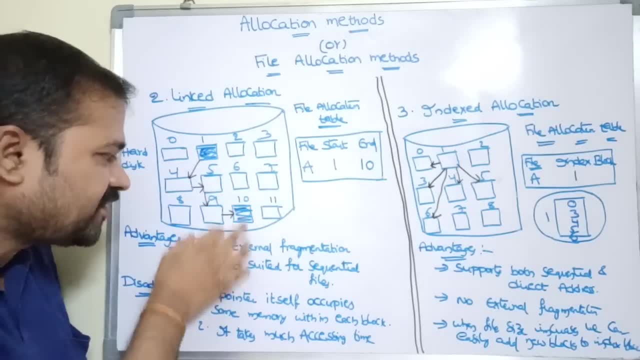 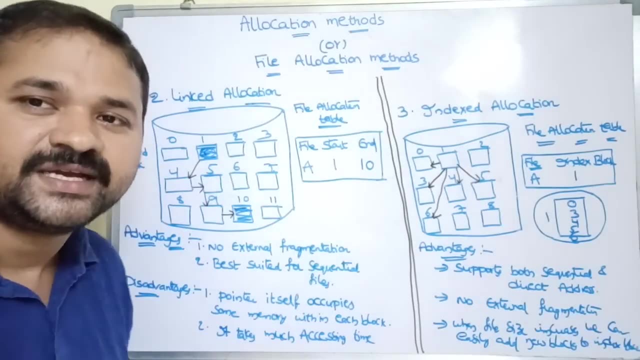 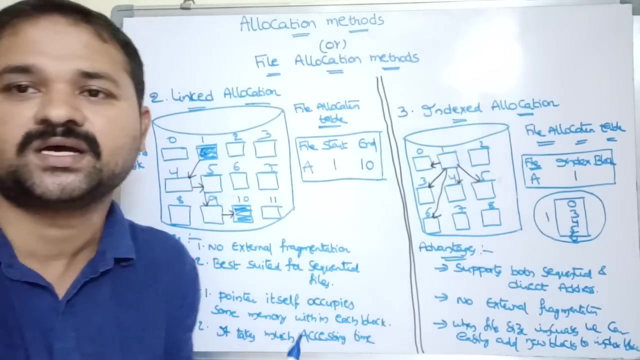 is a free block, then simply we can establish a link from that block to that block. So there is no external fragmentation here. And the second advantage is it is best suitable for sequential file, because sequential file means we can access the records one by one. So it is best suited for 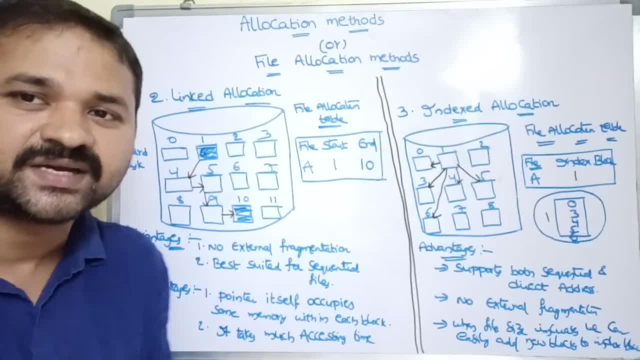 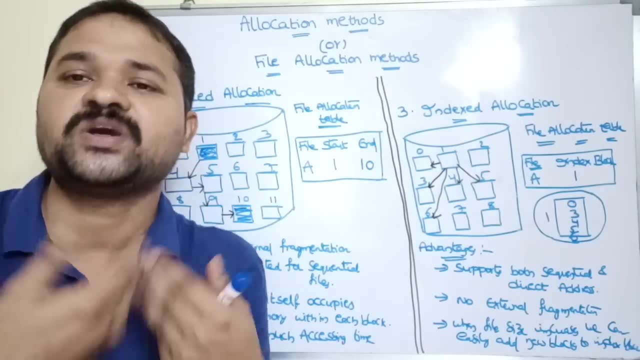 that approach. Let us see the drawbacks. The first drawback is here: in each block we have to maintain a pointer, So we need to store the pointer. In order to store the pointer, we require much amount of memory. And the second problem is it will take more amount of time in. 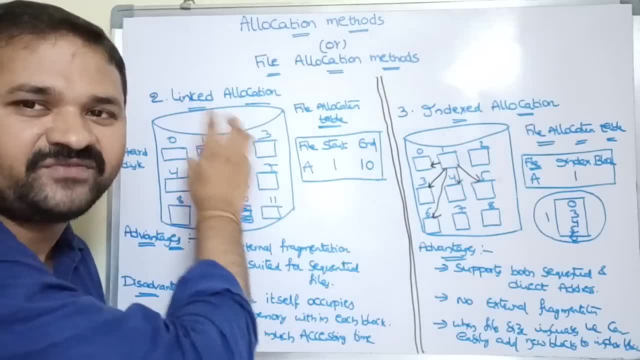 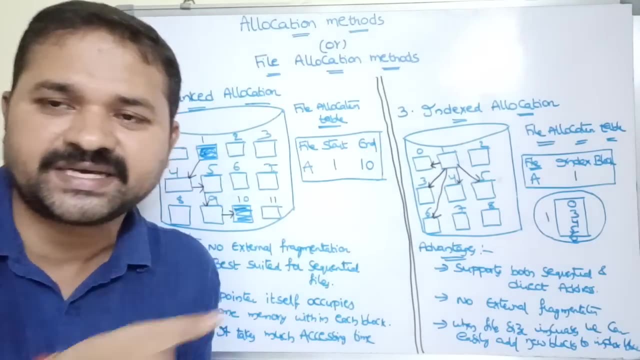 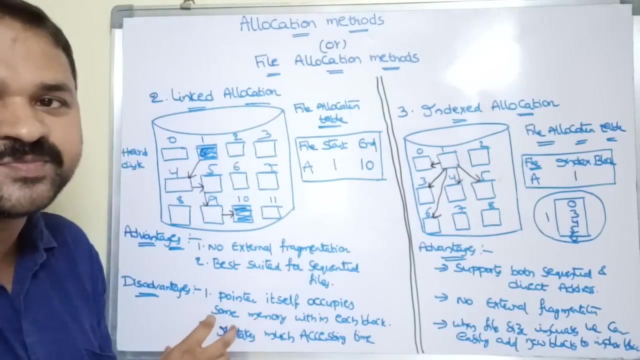 order to perform the traversing. Let us assume that here we have a link list with 100 blocks. If we want to access the last 100 block, then we need to access all its previous blocks. that is nothing but 99 blocks. So for accessing it will take more amount of time. So we can overcome these. 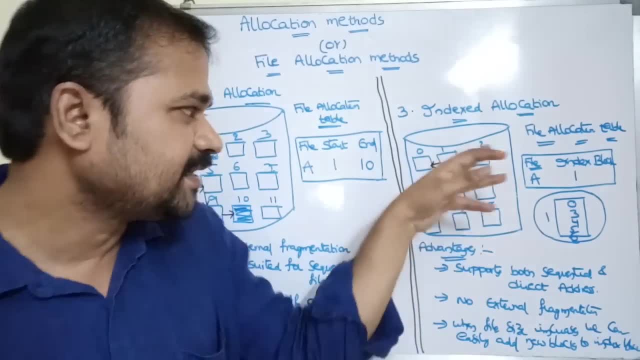 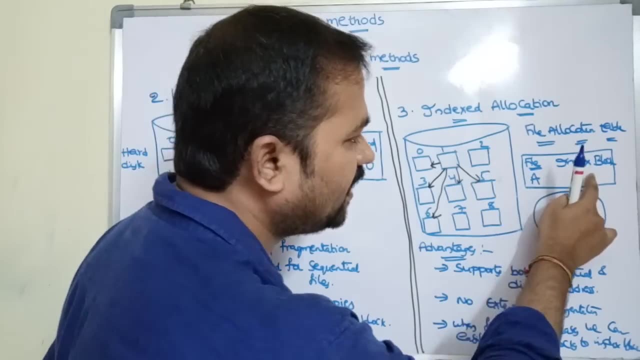 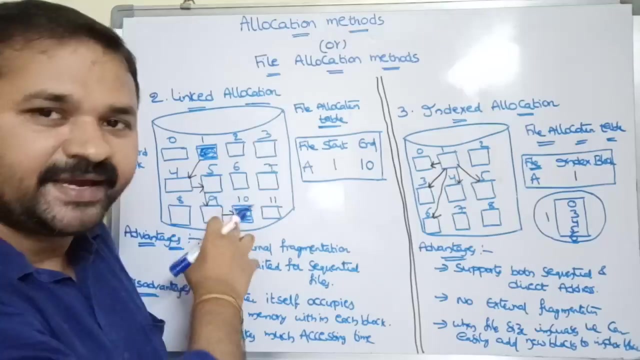 problems. The third approach is index allocation. Here it is based upon index block. Let us observe the file allocation table. Name of the file is A Index block is 1.. Now this block number contains the addresses of all the blocks here. If you take link list, then first block contains address of. 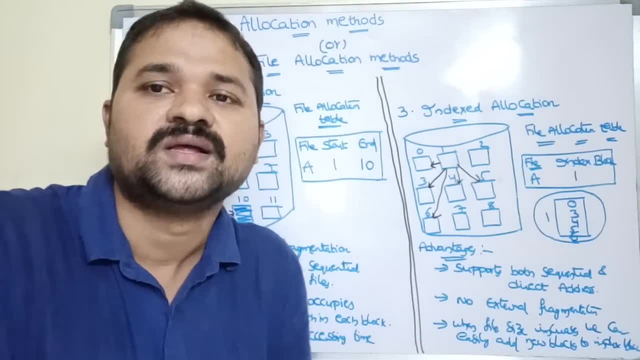 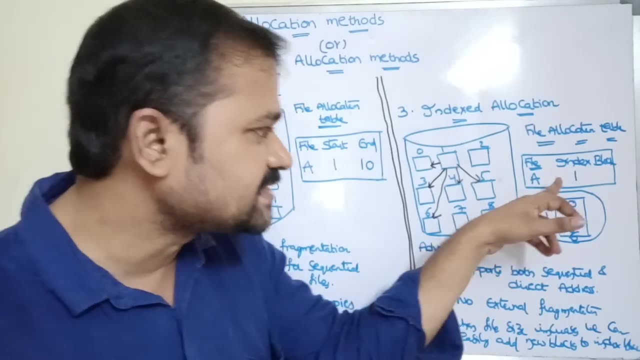 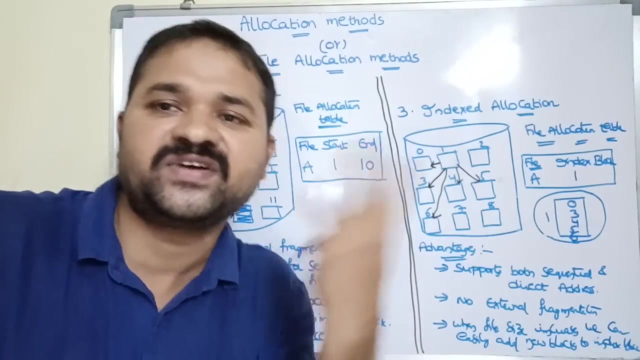 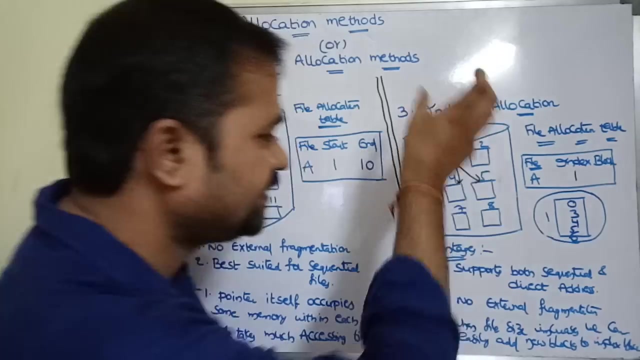 second block. Second block pointer field contains address of the third block. Third block pointer field contains address of the fourth block. If you take index allocation, a single block contains addresses of the blocks which are allocated for that file. So here this is nothing but index block. So index block contains the block. 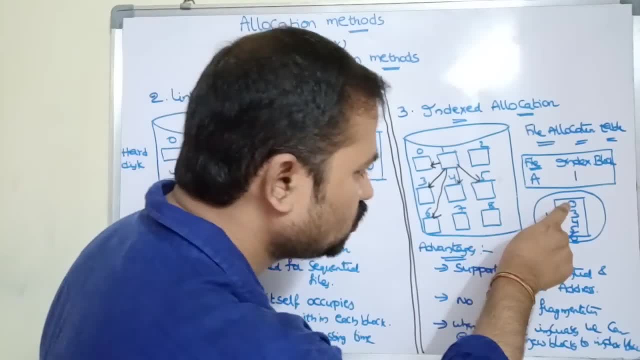 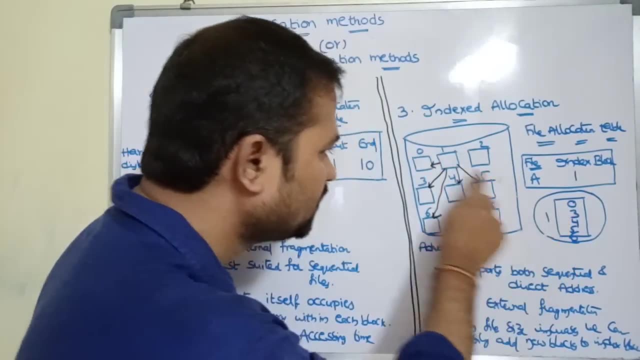 numbers which were allocated by the file. So the first block here is 0. So from 1 to 0, we have a link. Next block is 3.. Here, what is the index? block 1.. So from 1 to 3,. 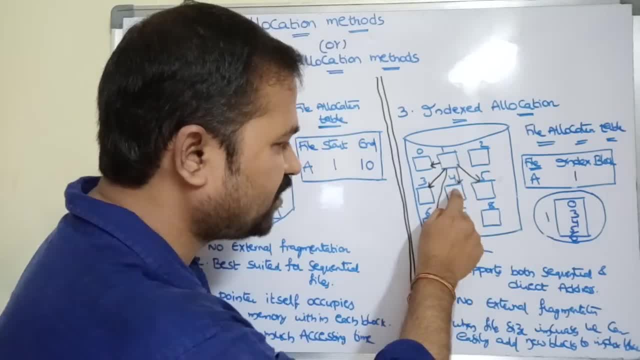 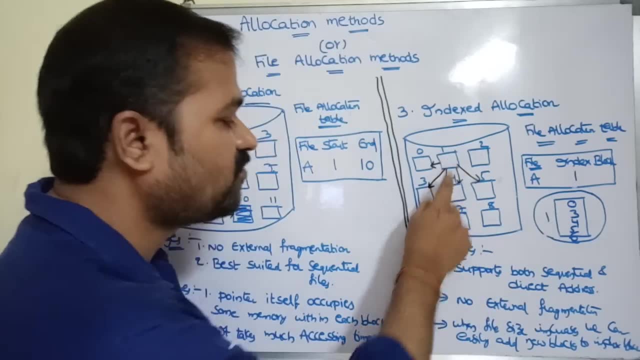 we have a link. Next block is 4.. So from 1 to 4, we have a link. Next block is 5.. So from 1 to 5, we have a link. Next block is 6.. So from 1 to 6, we have a link. So this is nothing but index.